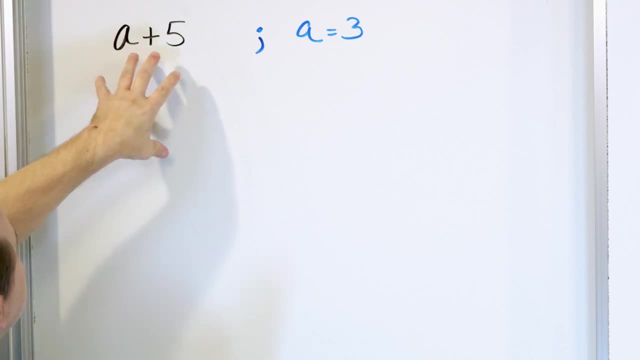 in math it just means calculate, calculate something. So here I'm giving you the expression a plus five and I want you to calculate or evaluate this expression if I tell you that a is three. Now, in real life, when we write real problems, we don't really know the value of a like, like going. 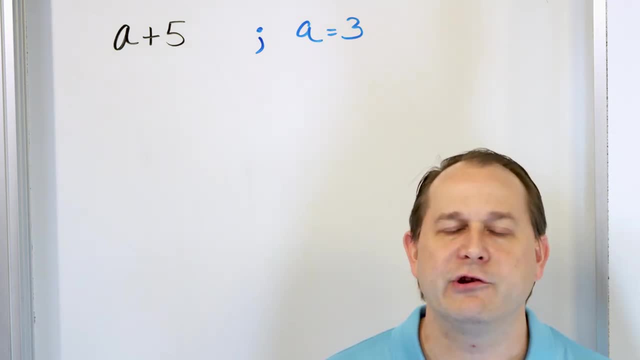 to the lakes or the gravity around the black hole or the temperature inside of a jet engine or something like this. We're trying to calculate and find those things. but here, before we get to that level, we're just trying to practice with using a variable. So here, if I tell you a is three and I 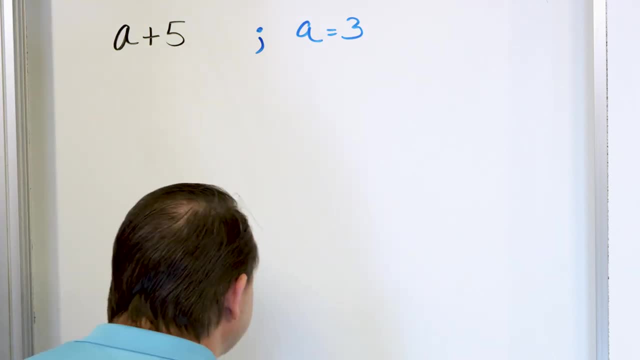 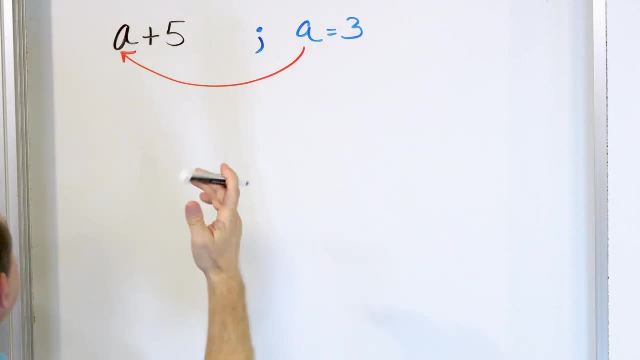 tell you the expression is a plus five. all you really have to do is take the value of this variable in and stick it in this location and calculate. So what you really are going to say is that this is going to be equal to the value of a. 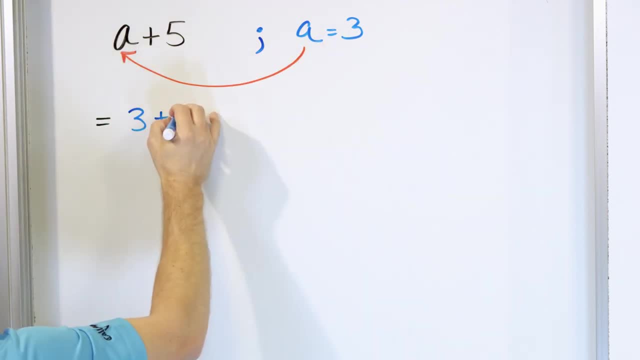 And for three, we're going to stick it right in here. we're going to say three plus five and then we're going to say that that's equal to eight and this is the answer to the question, because this is not a fully baked problem like we're going to get to down the road. I'm not asking you to calculate. 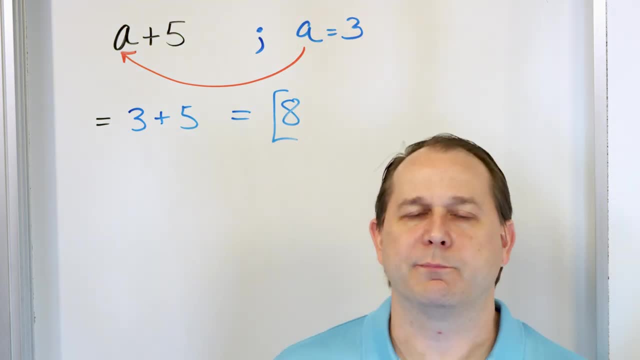 you know, I don't know the, the gravity around another planet or something like that. I'm not asking you to to do a full-blown problem. I'm just telling you that whatever a is, we're going to add five to it and now that I tell you the value of a, you can then calculate by putting it in there in. 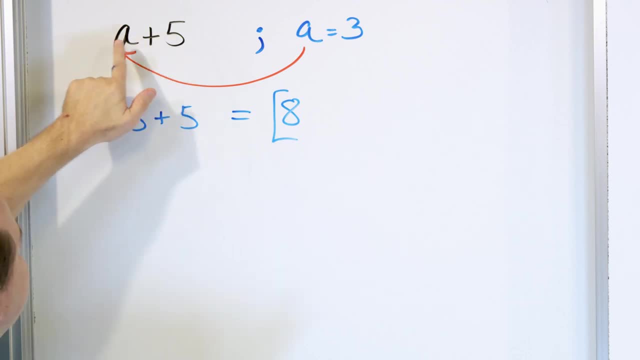 substituting in and you, and then you tell me what the answer to this expression is if a is in fact equal to three. So in this lesson we're going to get practice with that and the expressions are going to get a little more complicated with each step. but they're not. they're never going to be. 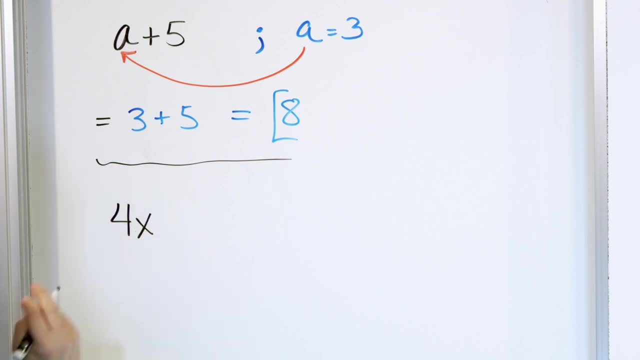 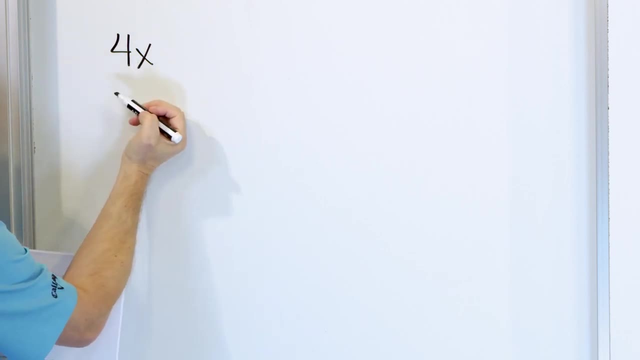 very, very hard. So let's say you have the expression four times x. So as we've said in the past, when you have a number next to a variable, even though there's no multiplication symbol between it, you assume that they're multiplied together. A number times a letter means a. 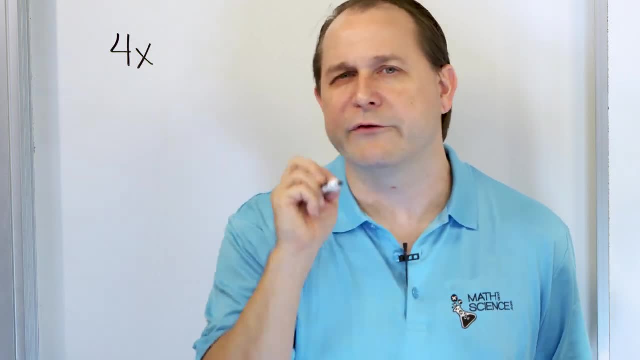 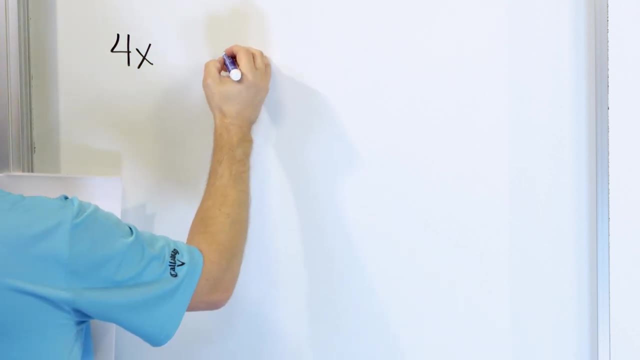 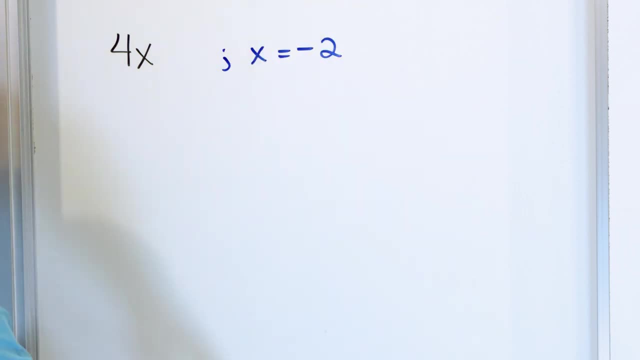 give to you that x is equal to negative two. So what you have to do is then take this value of x- and I'm telling you x is equal to- and stick it into this location here. So, because they're multiplied together, you could write it like this: four multiplied by negative two. but you see how. 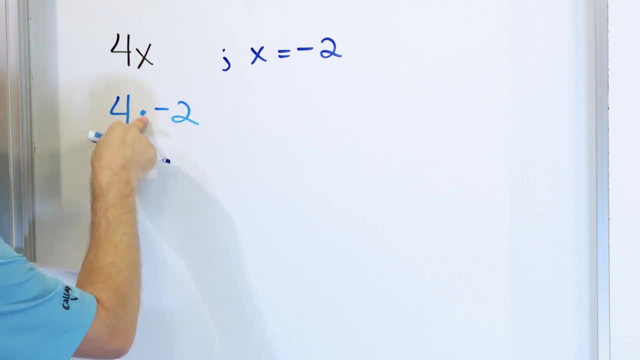 this looks kind of weird. They are multiplied because you're putting a dot here. First of all, you have to put something, if I, if you put negative two there, even though they're written next to each other, it looks like four minus two. that's not right. You could put a dot there showing their multiply, but that doesn't. 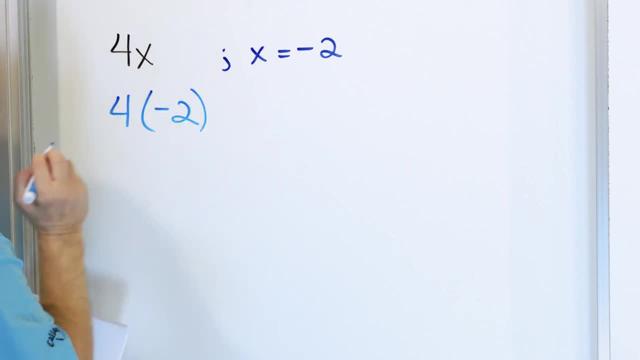 look so clear, It's probably easier to just wrap one of these in parentheses. So I like to go ahead and put parentheses around when there's a negative symbol there, because then it tells me that the negative two is multiplied by four. Now we've already learned how to multiply and divide, and 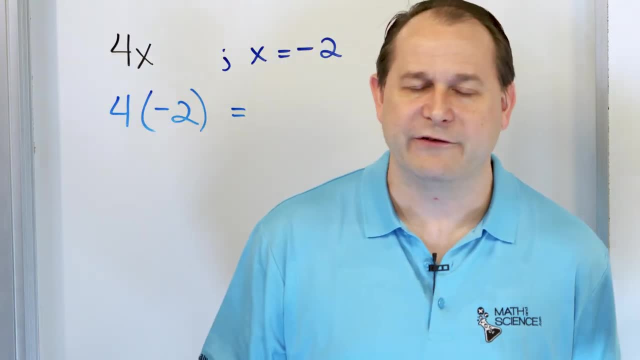 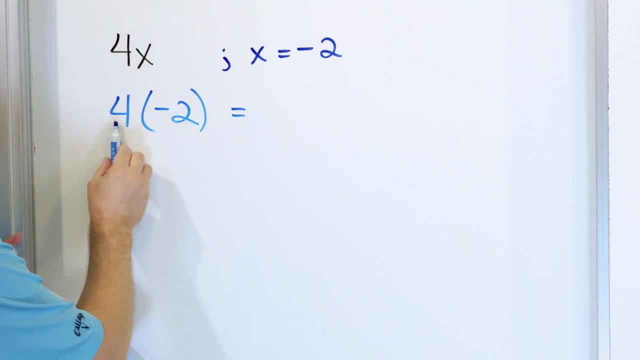 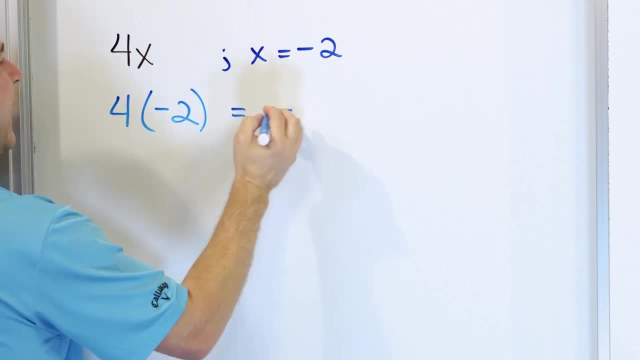 times negative two. So, because the signs are different, the answer is negative. and then four times two is eight. and so the answer to this expression: four x. when x is negative two, the answer is equal to negative eight. All right, moving right along to the next problem, Let's take a look. 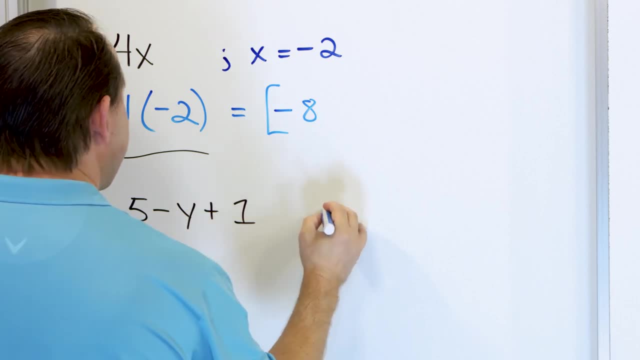 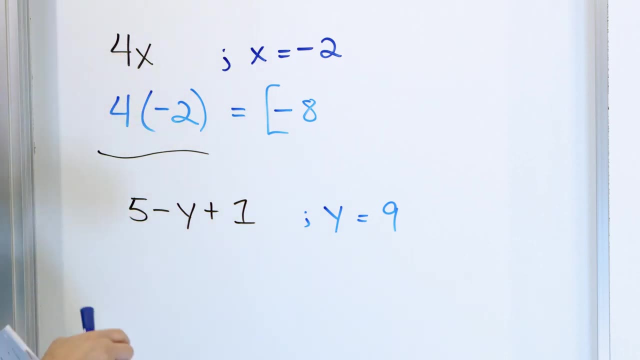 at this problem. So you've got negative four plus one and I'm going to give you that y is equal to nine. That's given to you and what we want to do is evaluate or calculate this expression here. So it needs to go right into the y position. So you say that that's five minus and then the nine goes right. 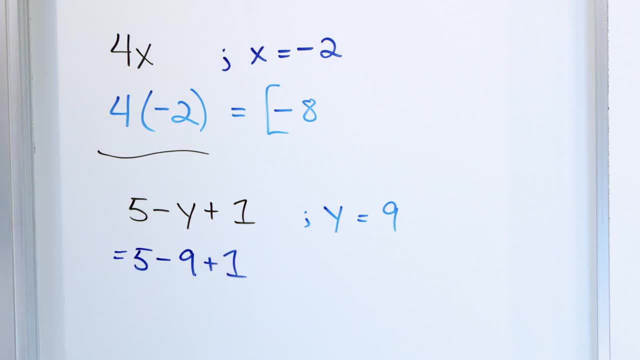 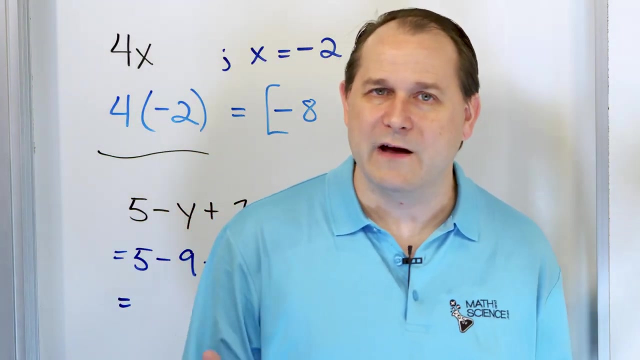 in there plus one. Now you have to use order of operations. There's no multiplication or division, so we don't have to do that. So we do addition and subtraction from left to right. So forget about the one for a second. What is five minus nine? So we've already done addition and subtraction of. 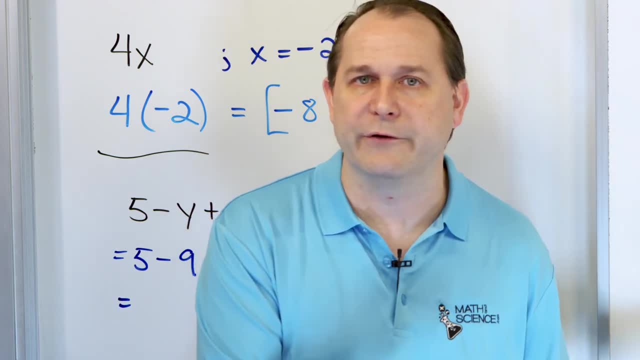 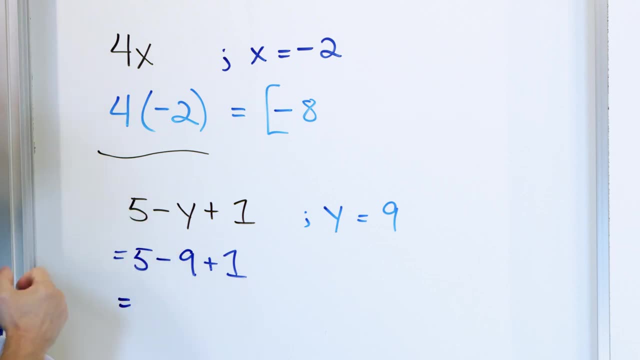 negative and positive numbers. Now you see why we have to master that. first, because I'm asking you to be able to do this. Five minus nine- you can think of it as five plus a negative nine, if you want to, And what you're going to do is subtract these numbers. Nine minus five is going to be four. 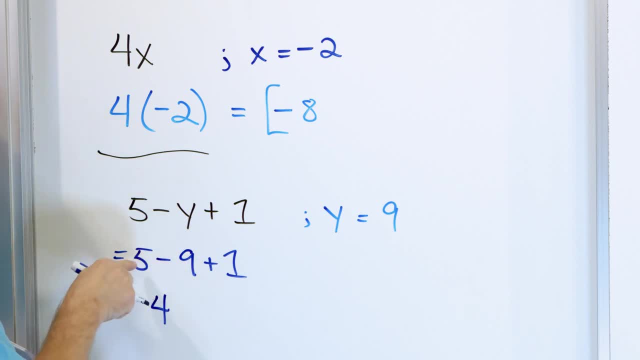 and the sine goes with the larger absolute value. This positive five is the absolute value of five. This, as a negative nine is a absolute value, is larger, And so you subtract the numbers and the sine goes with the larger absolute value. So five minus nine comes out to negative four. 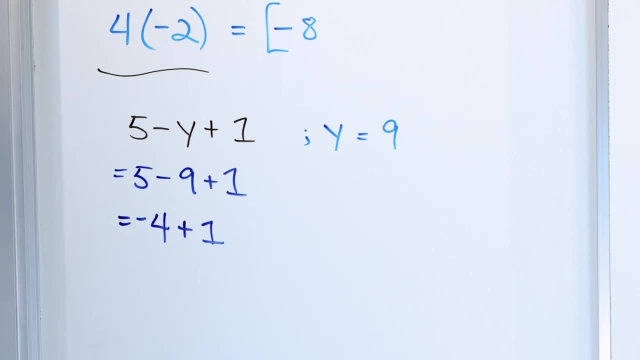 but we still have to add this one to it. All right, So the next step here is to take a look and solve this Negative four plus one. Again, the signs are different When we have opposite signs and we're adding them together. we just subtract the numbers. Four minus one is three. 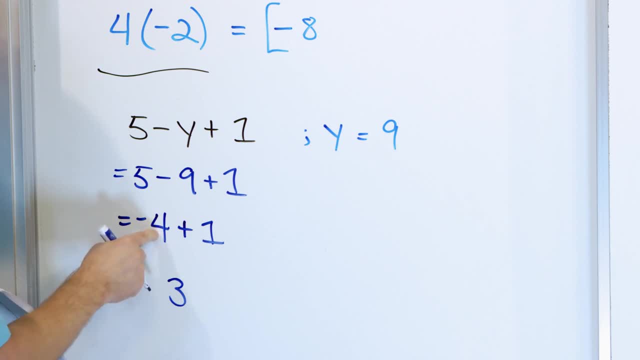 And the sine of the answer goes with the bigger absolute value. Negative four plus one. Negative four has a bigger absolute value, So the sine goes with it And the answer is negative three. If you don't like that, you could just flip it around and write the positive one here. 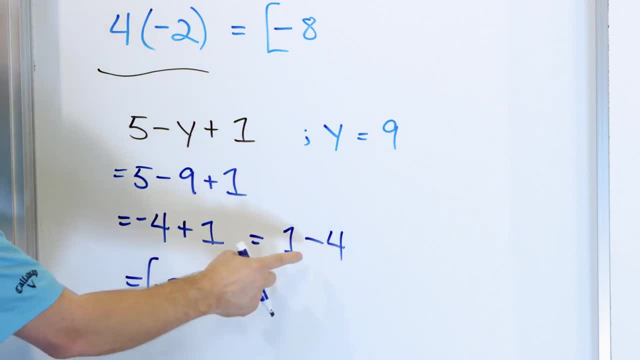 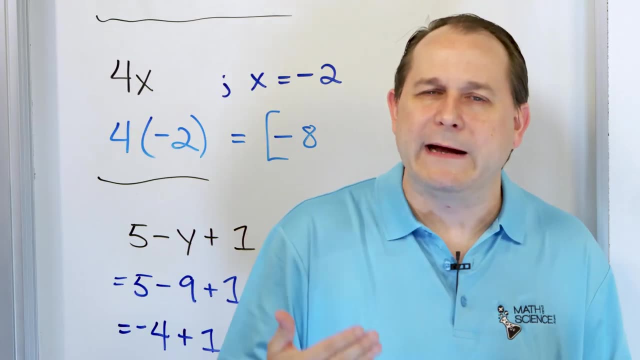 minus four and make it one minus four. So one minus four is the same as negative three, And it's also the same as negative four plus one. Again, I'm kind of not explaining every single thing about adding and subtracting these integers, because we've already covered it in great 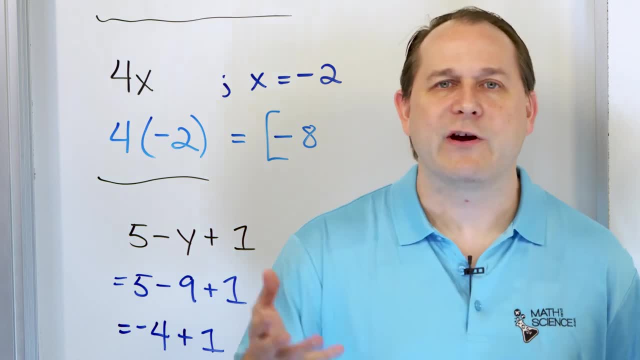 detail And it's very important that you master adding and subtracting negative three And if you don't like that, you could just flip it around and write the positive numbers and multiplying and dividing negative numbers. If you haven't, then please go back and 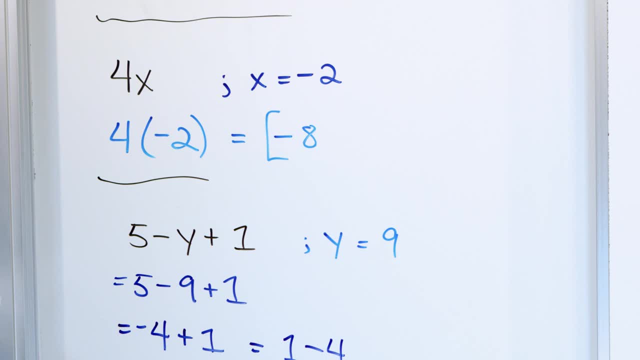 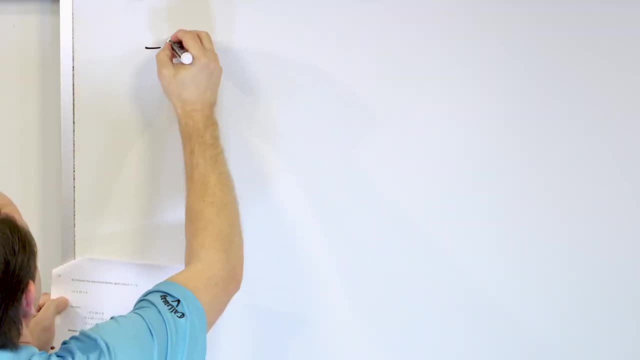 practice it, because you have to use that skill- It's like walking- before you can do anything else. All right, Let's take a look at problem number four. What about negative two? And we're going to add to that 20. And I'm going to divide by b And I'm going to tell you: 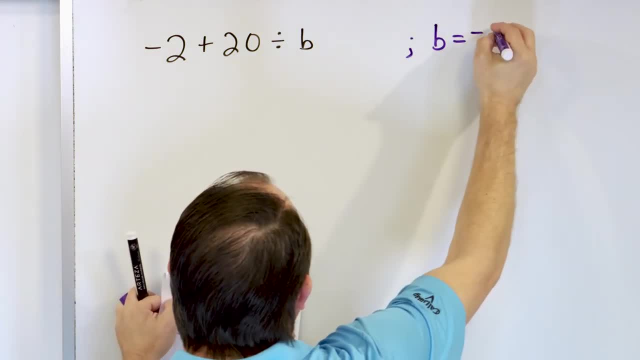 or give to you that b is equal to negative five. So, given that b is equal to negative five, So I'm going to add to that 20. And I'm going to divide by b And I'm going to tell you or give to: 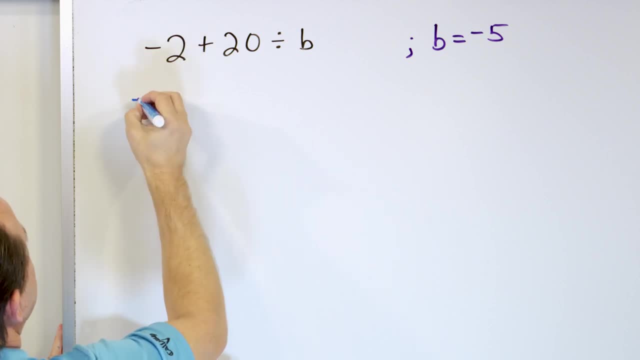 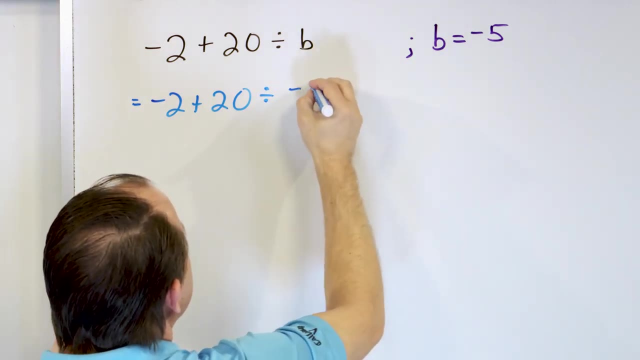 you that b is equal to negative five. So what you do is you stick negative five into this location right here. So we rewrite it: negative two plus 20. And then we divide by And then, since there's a negative sign, you could leave it like this: I guess it's kind of readable, but it's just. 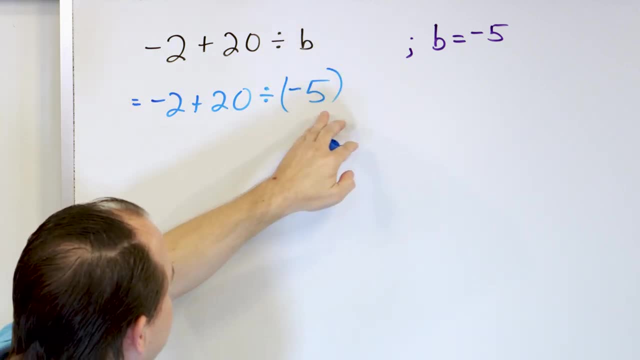 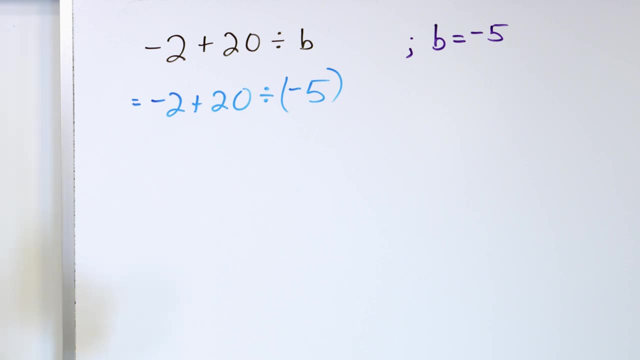 a little easier if you wrap your negative numbers around with parentheses so that you don't get lost and you don't accidentally overlook the negative sign here. All right, So here we have to calculate the answer. We have to use order of operations. Remember, for order of operations, just a quick. 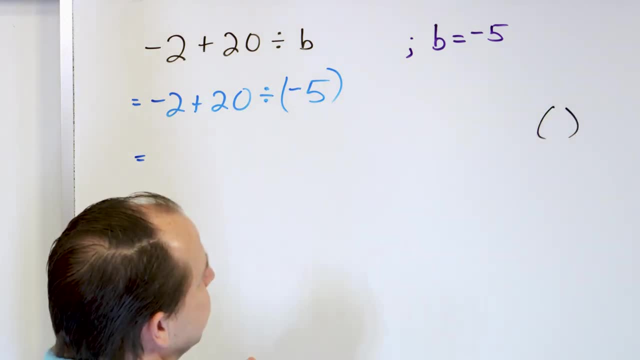 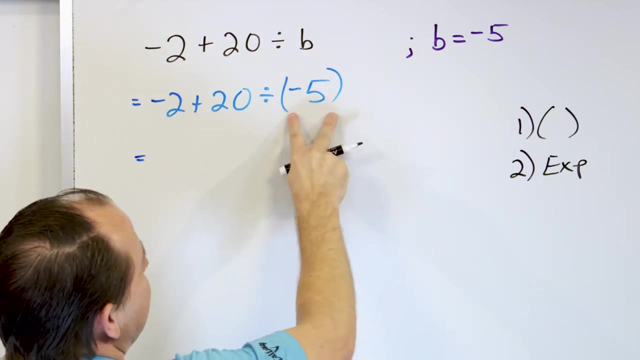 review. The very first thing we're going to do is we're going to add to that 20. And we're going to do any parentheses first, right, And then the next thing you look for is any exponents. We don't have any exponents here. We do have parentheses, but the only thing in there is a number. So there's. 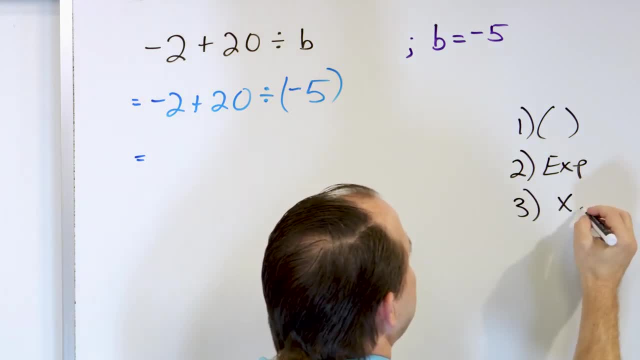 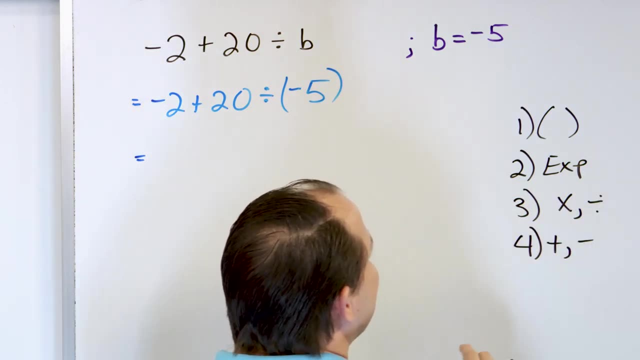 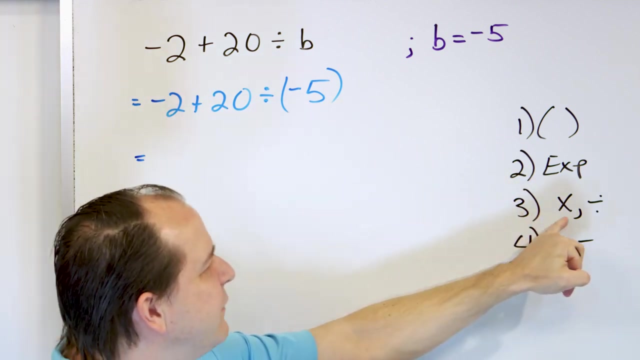 nothing to do. And then at the third priority level we multiply and divide from left to right, like this: And in the fourth priority level we add or subtract from left to right. So we really we do have parentheses, but there's nothing in there, There's no exponents here, So we have to. 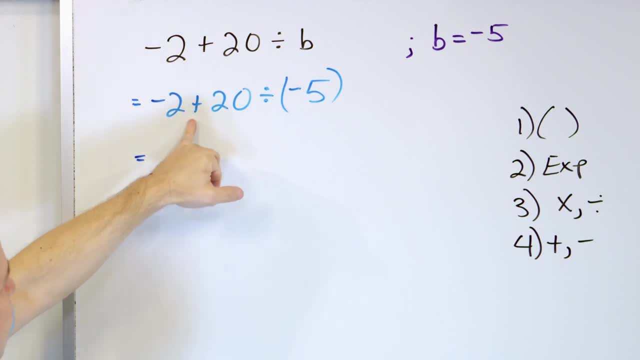 do any multiplication. So we're going to do any multiplication And then we're going to do any multiplication and divisions first. So we do not do this addition. You do not do this addition first. You must do this division first. So what you're going to have is the negative 2 stays the. 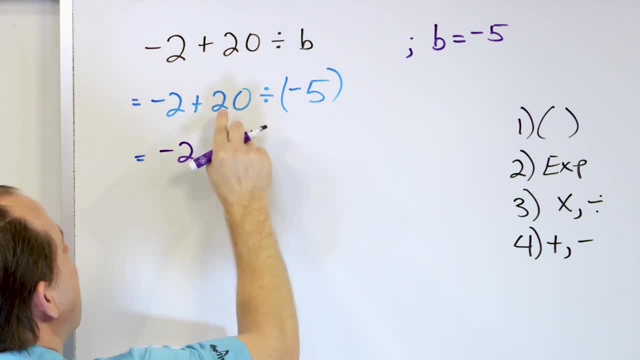 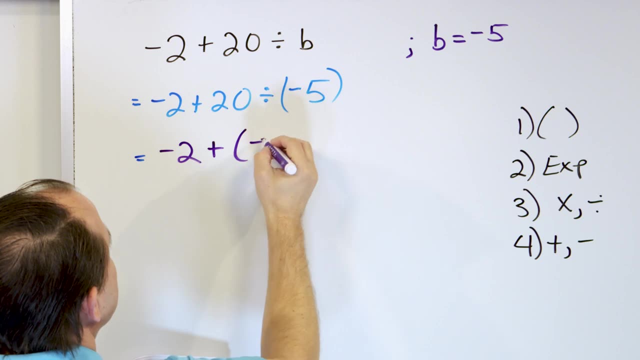 same. We have to take 20 and divide it by negative 5. Remember: positive divided by negative is a negative, And 20 divided by 5 is 4.. So write it as 2 plus a negative 4. So the plus sign comes. 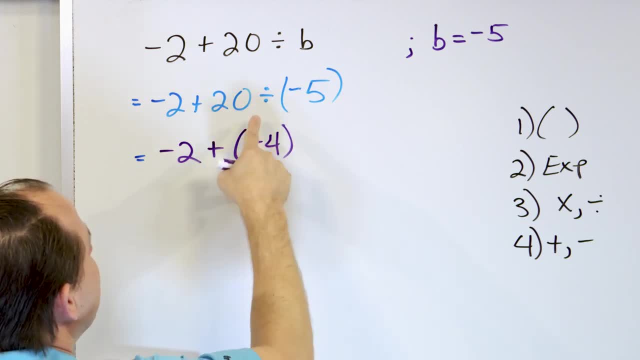 from here, And now we're doing this here, We get a negative answer Again. you don't have to put the parentheses. You could just write it as 20 plus a negative 4, I guess. But usually wrapping it in parentheses is a little clearer what you have here. 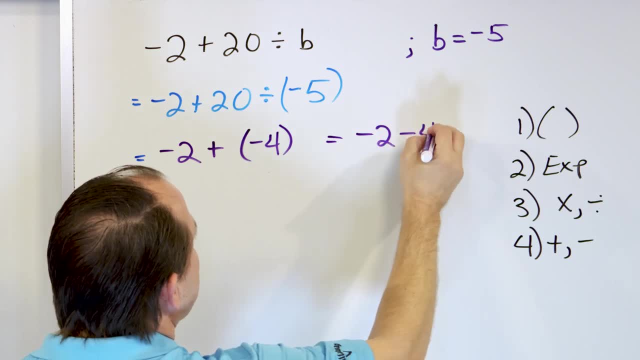 And you could say, if you wanted to, this is negative 2 minus 4.. Remember, plus a negative is the same as a minus sign. So if you like to read it like this, it's fine. If you like to read. 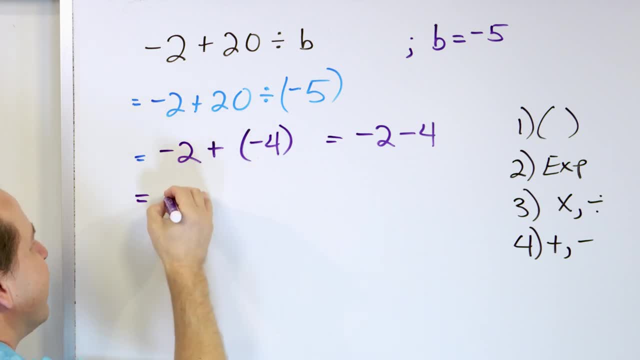 it like this. it's fine Either way. when you have a negative plus another negative, the answer is negative. 2 plus 4 is 6.. This is like $2 of debt And I'm adding four more dollars of debt, So I 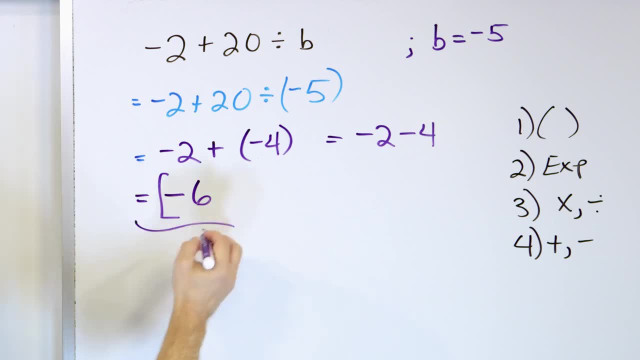 have a total of $6 of debt. So the answer is negative, 6. It's a simple problem, but also a tricky problem. A lot of students will accidentally add these numbers first and then try to divide, But that violates order of operation, so you get the wrong answer. So we're using skills from 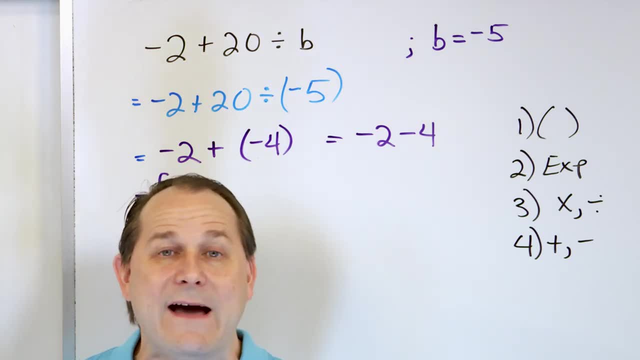 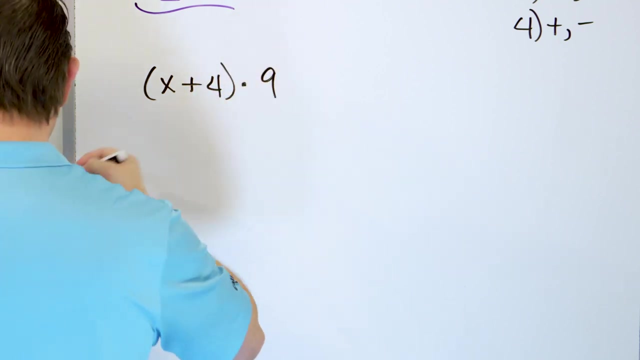 before. We have to understand order of operations, Then we have to also know how to add and subtract, multiply and divide these negative numbers integers. And we have to put all of that together. All right. next problem: Let's say we have x for the expression x plus 4. And we're going to multiply that by 9. And I'm 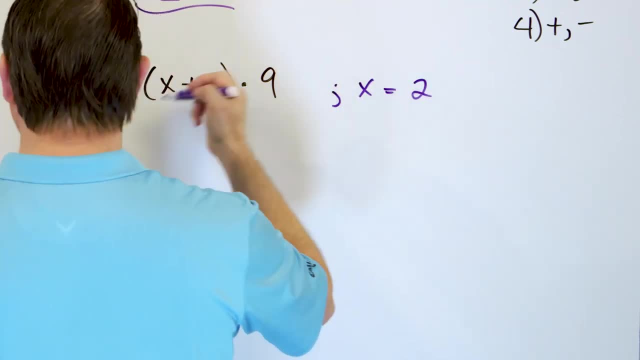 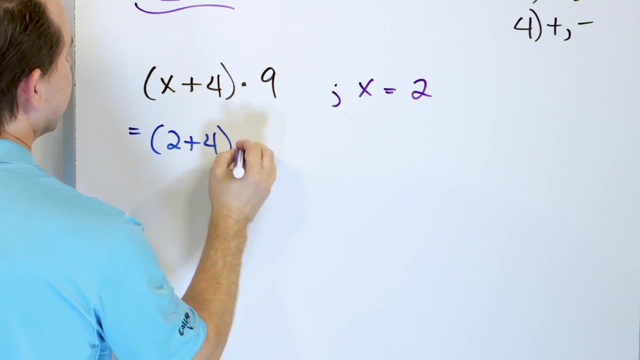 going to give you that the variable x is equal to 2.. So what you do is you stick 2 right into this location And you say it's 2 plus 4. And we're going to multiply that by 9.. Now order of. 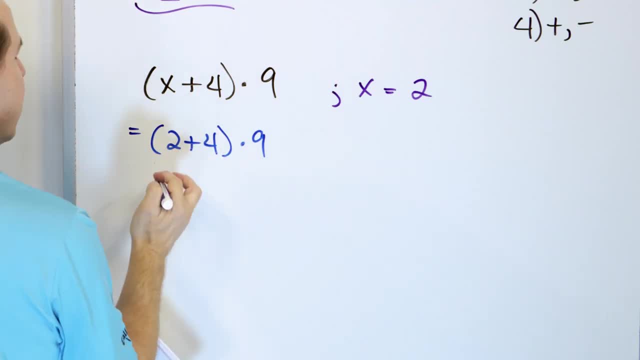 operations again says we do the parentheses first. So we say 2 plus 4, we do that first, That's 6.. After we calculate it we can drop the parentheses. We still have to multiply. And 9 times 6 or 6 times 9,, 54 is the answer Positive, of course. 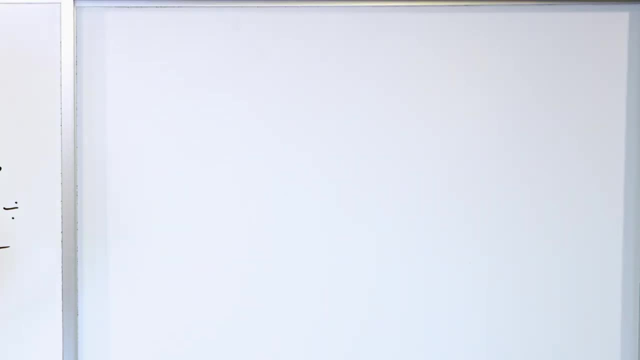 All right, we're halfway home, making good progress, But the expressions will get a touch more complex as we go throughout all of these problems. What about 4 divided by the variable a plus 9?? And I'm going to tell you this is not an a here. This is the number 9,, by the way. 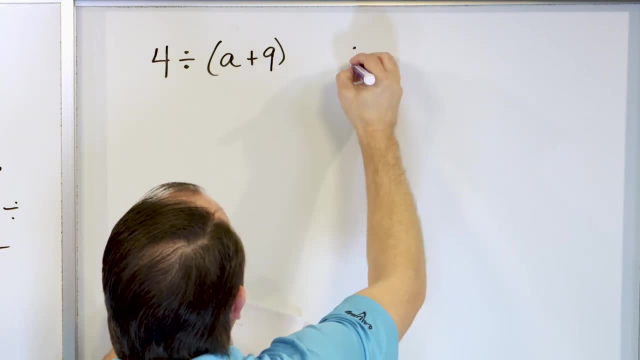 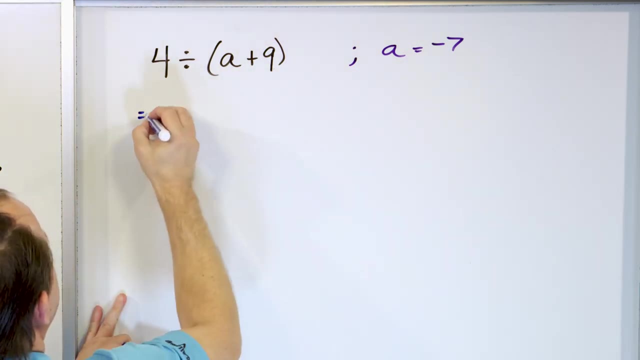 right here, This number 9, right there, And I'm going to tell you that the variable a is negative 7. So we have to stick it in here. So we have 4 divided by we have negative 7 plus 9.. You could wrap the negative 7 in. 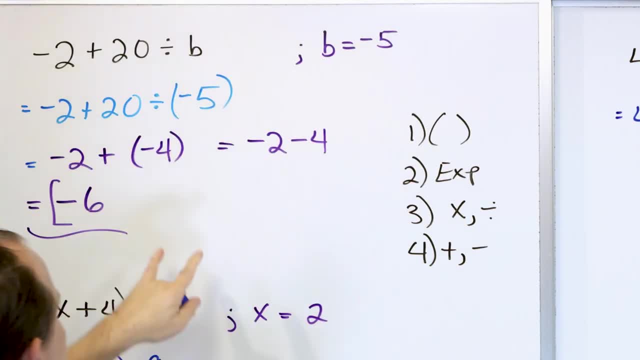 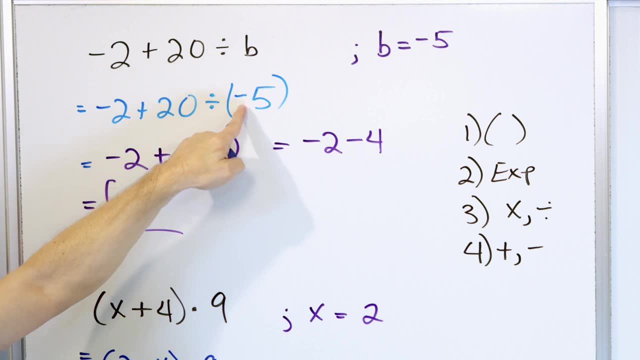 innermost parentheses, but I think this is pretty readable here. The reason I add it here is because if you put plus minus right next to each other, sometimes you overlook the minus sign. If you put divided negative, sometimes you overlook the negative sign, But I think here the negative 7. 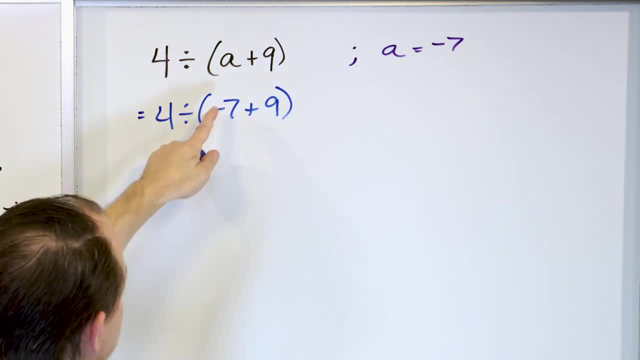 plus 9, it's pretty clear, So I don't think we need to, But you could wrap it in parentheses if you want. Now, order of operation says we have to do what is inside. if you're first, We cannot do this division first. So it would be 4 divided by what do we get when we calculate this Negative? 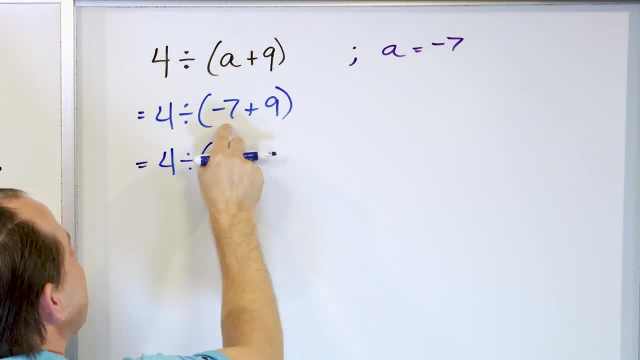 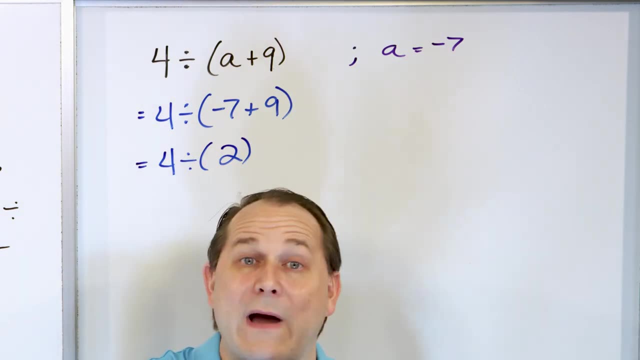 7 plus 9,. they're opposite signs. So what do we do? We subtract: 7 minus 9 is 2. And the sign goes with the larger absolute value, which is the 9.. Basically, when you add or subtract, when you add. 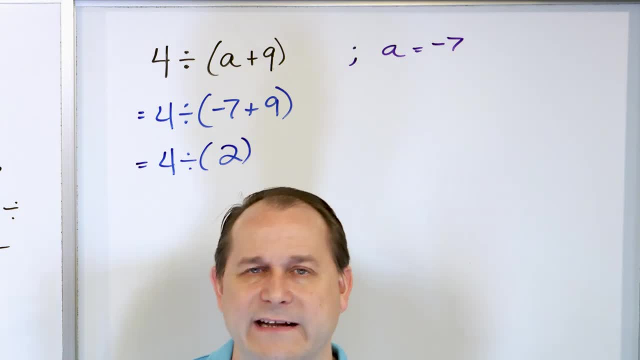 negative and positive. when the signs are different for the integers and you're adding them together, just subtract the numbers as usual, And the sign of the answer just goes with whichever one is a larger absolute value. So it's positive, And then finally we have 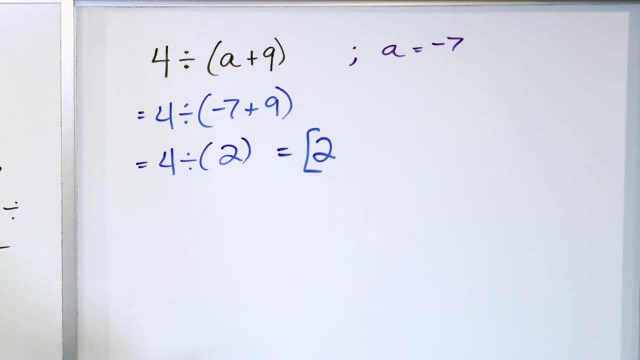 4 divided by 2, which is 2.. And these are both positive, So the answer also is positive. All right, let's take a look at problem number 7.. y plus 2y 2 times y minus 5.. Now this is: 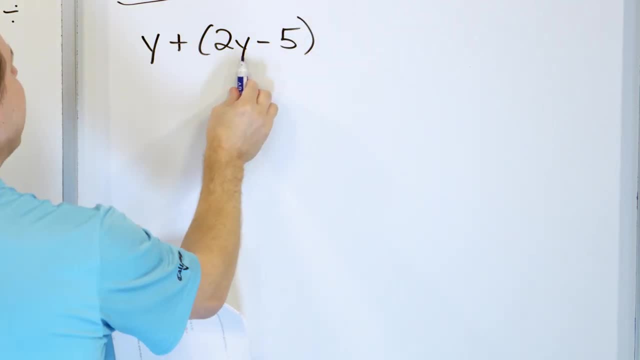 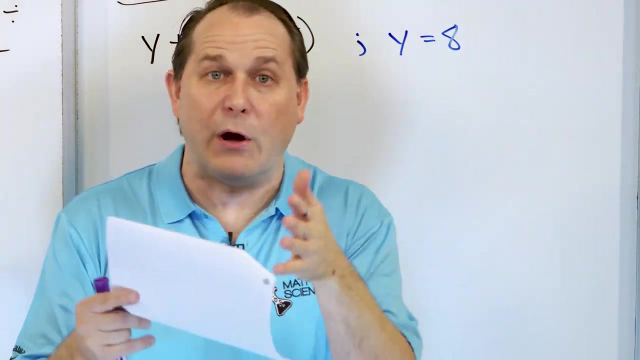 the first one of these expressions, where we have the variable in two different locations And this value of y, I'm going to tell you, is equal to positive 8.. Now, if you see a variable y in two different locations, don't stress out about it, It just means that that variable is involved. 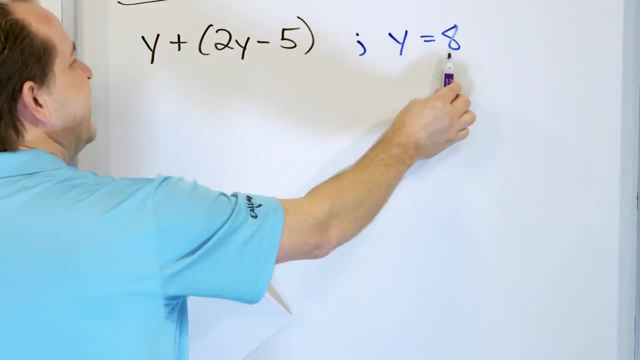 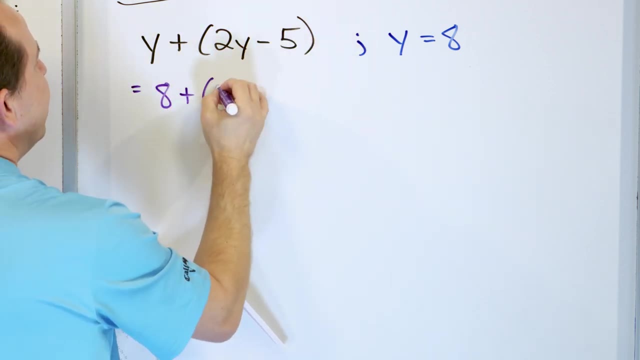 in two different parts of your calculation, But you still put the same value of 8 in both places, because y is in both places and the value of y is 8.. So we say it's 8 plus 2. Now we have 2 times. 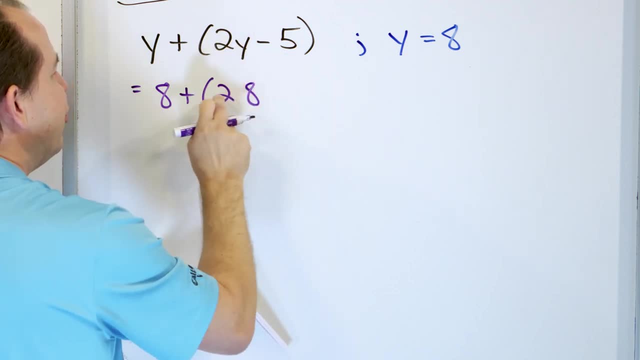 8. You have to put some kind of multiplication here to show you can't just put a 2 and an 8 together. That leaves us with 2 times 8.. So we have 2 times 8.. Now we have 2 times 8.. You have to. 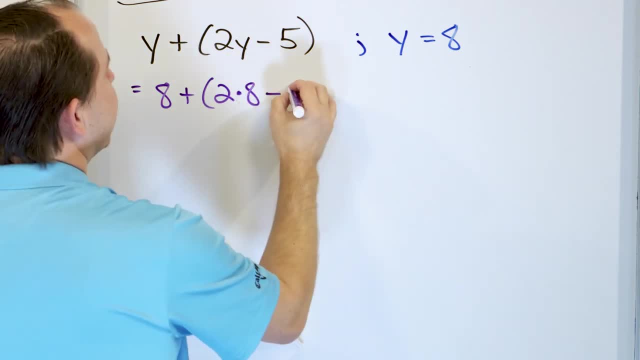 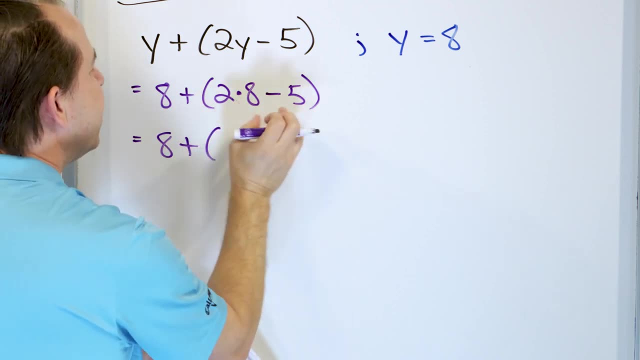 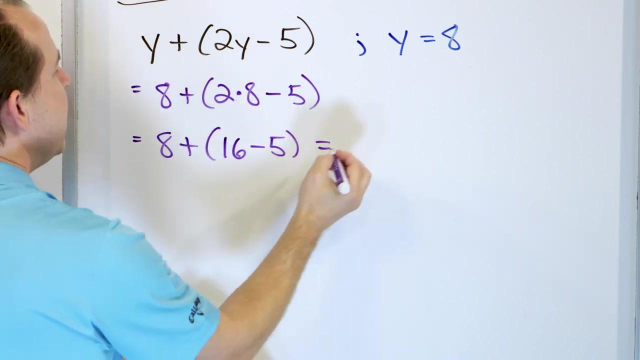 put a dot there and then minus 5.. So you just substitute there. Now what do you do? You have to work inside the parentheses first, But inside of here you have multiplication and subtraction. You multiply first, 2 times 8 is 16. You still have to subtract that 5. And then you have on. 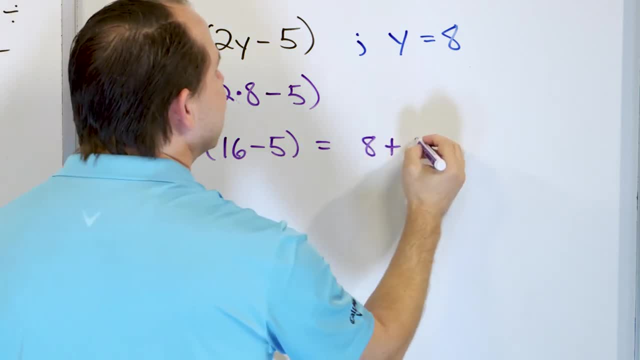 the inside of the parentheses. you have to finish the inside first. 16 minus 5 is 11.. Now we can drop those parentheses And 8 plus 11 is 19, positive 19.. And that is the final answer. 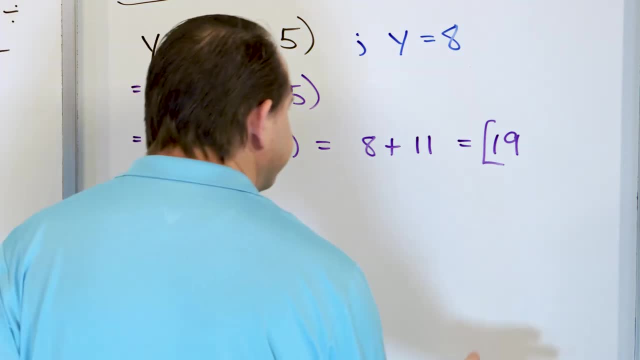 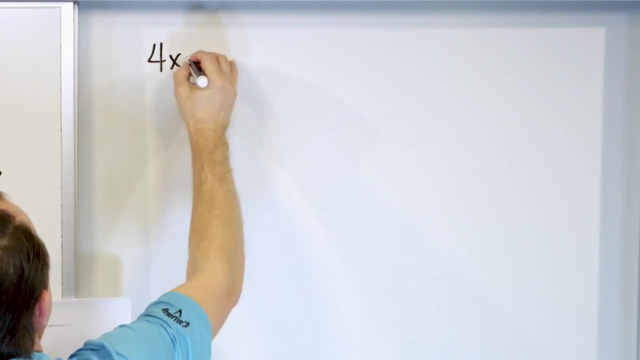 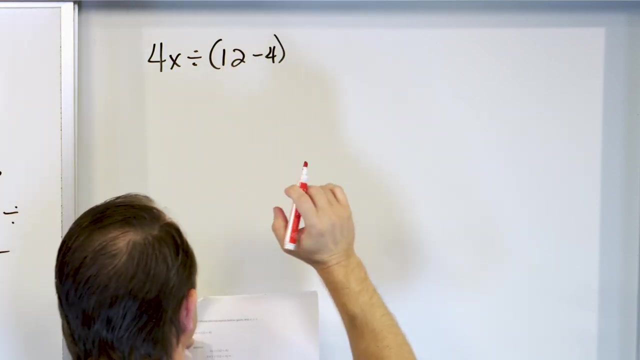 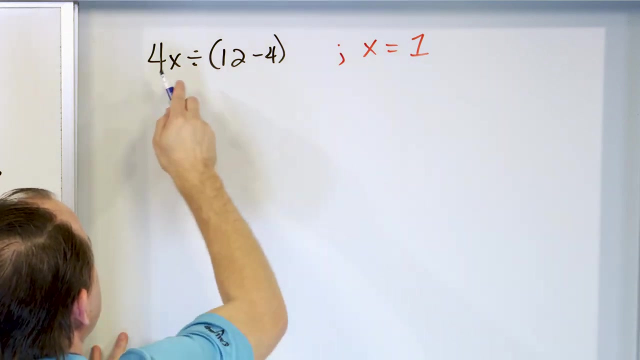 All right, Only three more. What about 4 times x divided by 12 minus 4?? And I'm going to give you that the value of x is equal to positive 1.. So you stick the value of 1 everywhere you see an x. 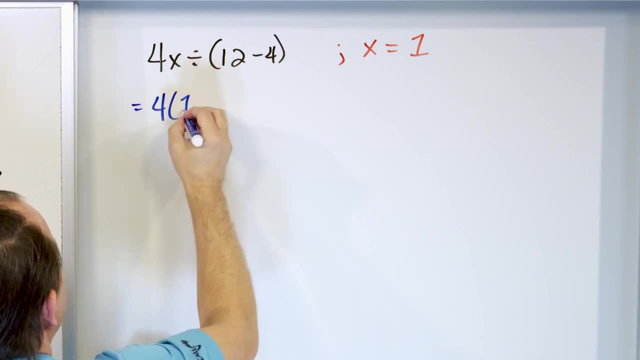 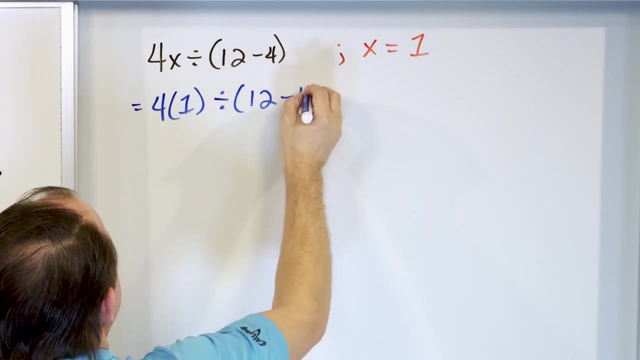 So here we have 4.. This is going to be times. 1. You can put a dot in between. I'm going to wrap it in parentheses. do it whichever way you prefer. divided by 12 minus 4.. All right, So what we need to do next is inside the parentheses Here. 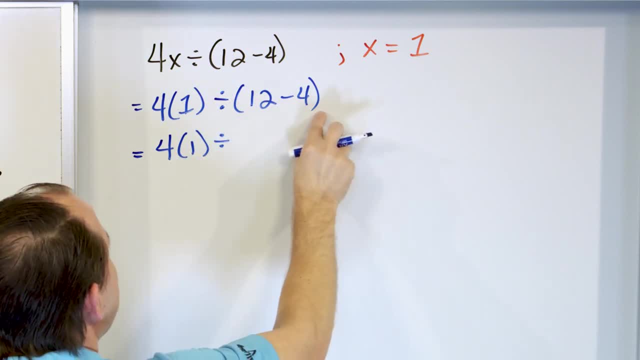 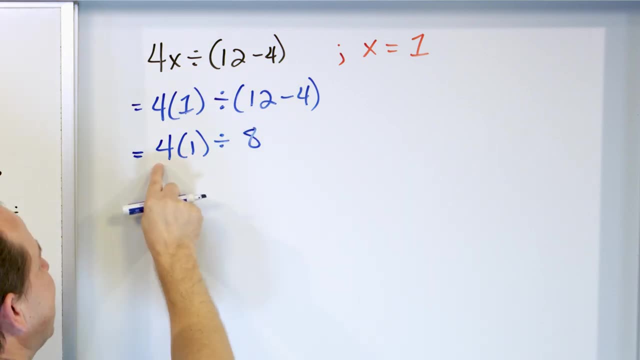 we still have a 4 times a 1, right, But inside we have to do this first: 12 minus 4 is what 8.. So we have an 8 here. So now we have multiplication And then we also have division. 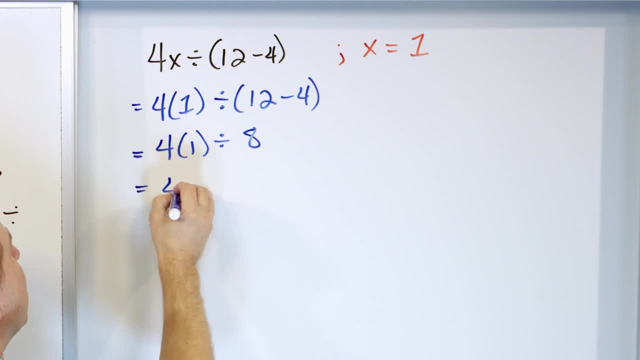 We do it left to right. So 4 times 1 is 4. And we have to divide by 8.. 4 divided by 8. Now you might not know what to do here, But then you realize this is the same as 4 over 8.. 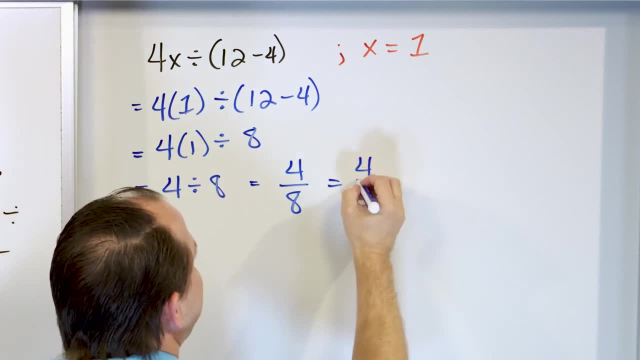 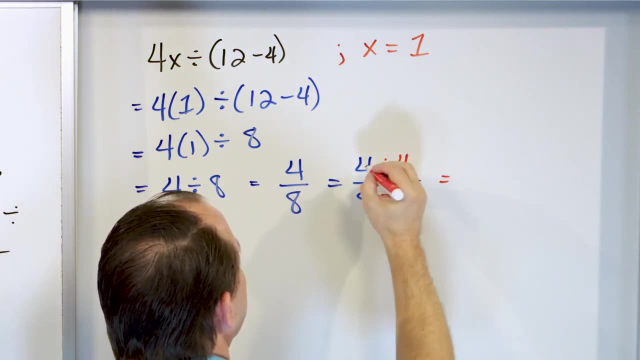 4 divided by 8 is 4, eighths like this, And so it's basically a fraction. We can simplify this fraction by dividing the top by 4 and the bottom by 4.. And 4 divided by 4 is 1.. 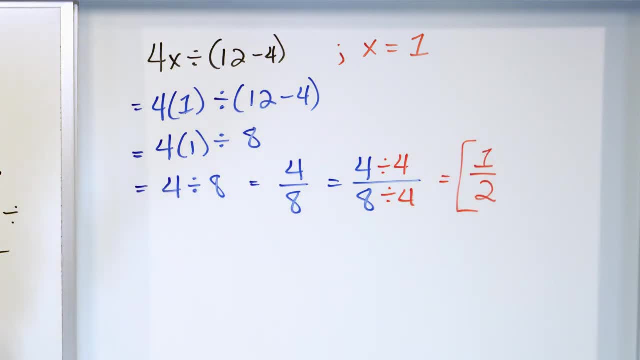 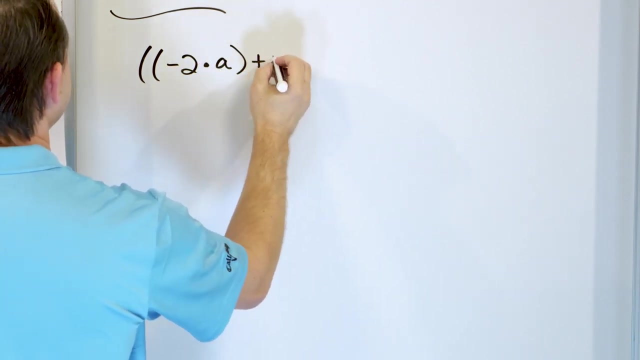 And 8 divided by 4 is 2.. So once we put a value of 1 into this expression, we calculate an answer of 1 half back. All right, Next problem: Let's say we have negative 2 multiplied by a, Then we're adding 10 to it, Close that off And then we're going to divide by a. 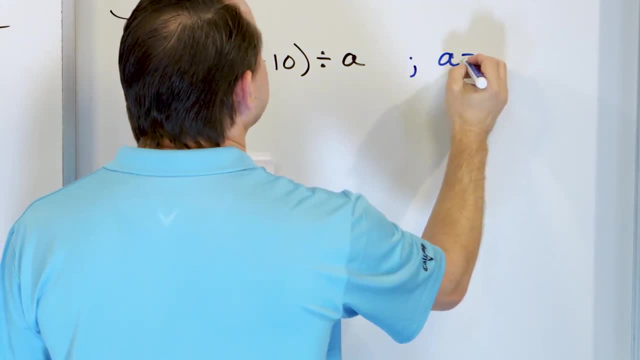 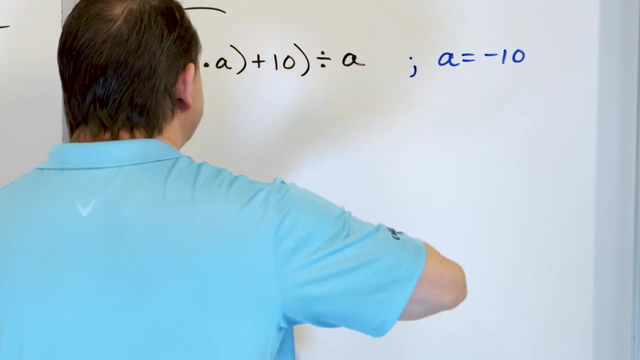 All right, Same thing. I'm going to also give you that a is equal to negative 10.. Now, because you're putting a negative number in here, you might have to put some extra parentheses to make sure it's readable, But that's really up to you. 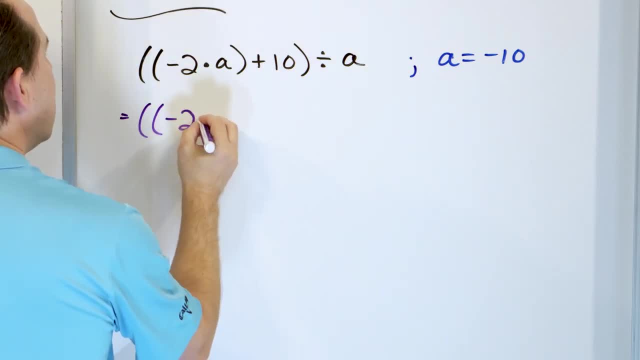 Here on the inside we have negative 2 multiplied by a. I could put a dot, you know- negative 10.. Like this, But it doesn't look so readable. So what I prefer to do is say it's negative 2 times 10.. 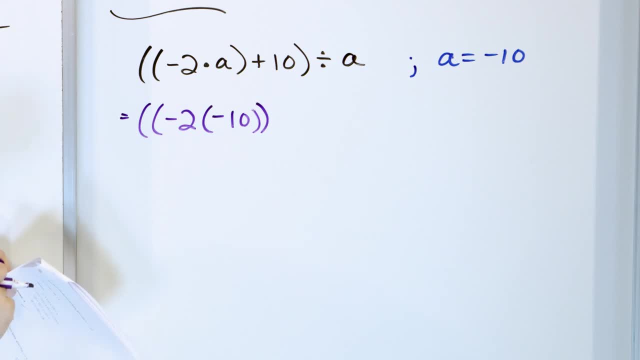 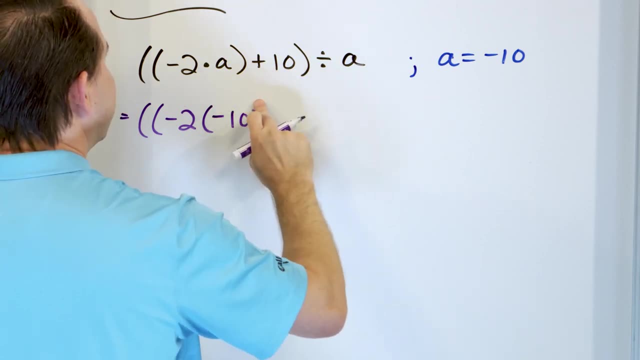 Let's see here: Negative 2 times 10.. Yeah, like this- And that to me is a little bit clearer- that they're multiplied together. But if you want to put the dot, you're more than welcome to here, And then we're going to take this out of parentheses off like this: 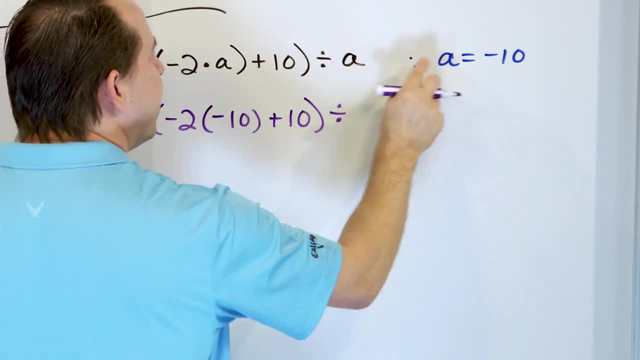 We still have to add 10.. I forgot about that. And then we're going to divide by what? By negative 10.. Again, you could put a negative 10 here, but it just reads a little bit clearer to me to put parentheses around it. 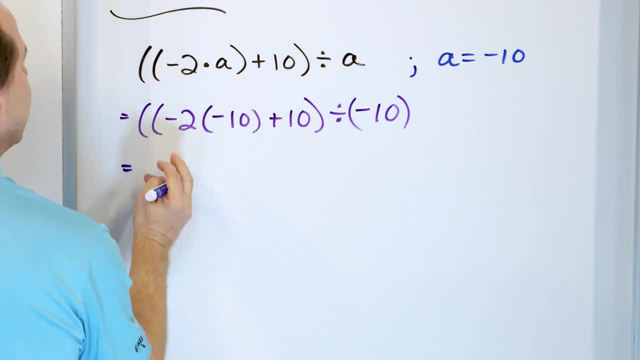 So next we look on the inside. We have to do what's inside of these parentheses. Inside we have multiplication and also addition. The multiplying happens first Negative times. negative is positive. 2 times 10 is 20.. So it's positive 20.. 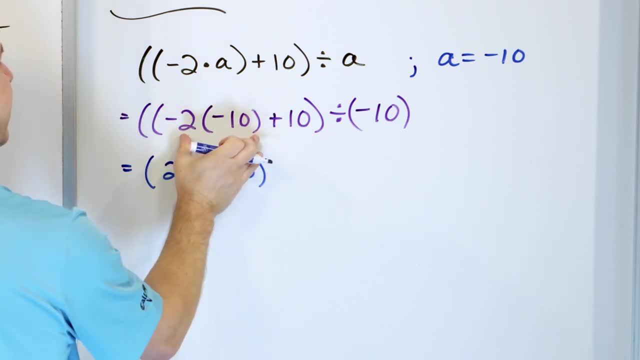 We still have this plus 10 here. So you see, once we do the multiplication here, then we can drop these parentheses here And we have divide by negative 10.. We still have to work inside of here. 20 plus 10 is 30..